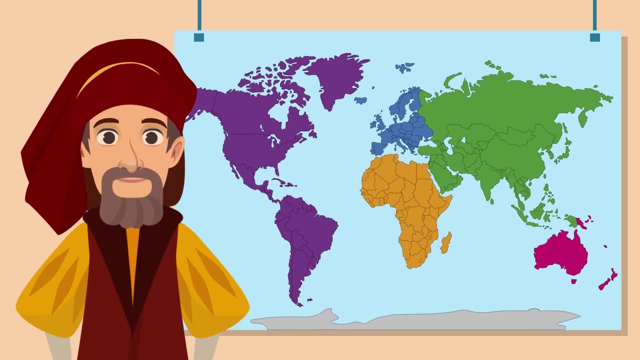 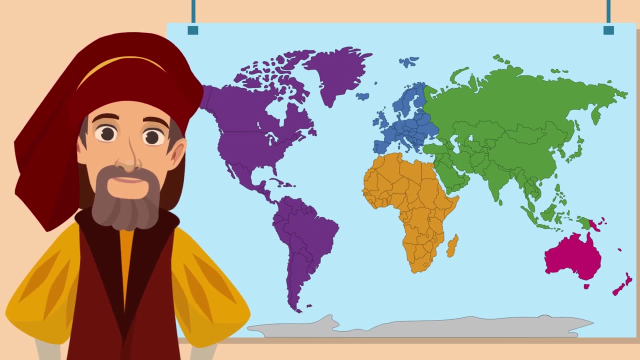 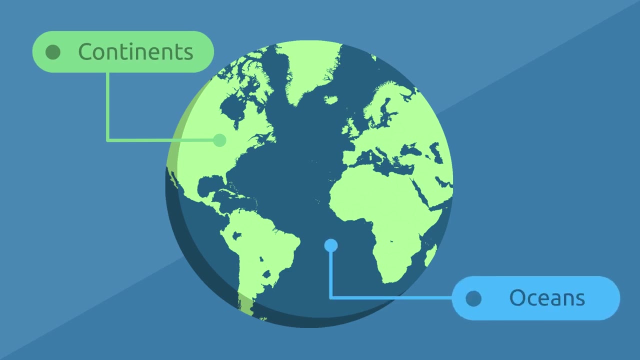 They don't have a clear answer. Well, while they're making up their minds, we're going to be following this map, which shows six continents. As you can see, the surface of the Earth consists of massive land masses separated by oceans. 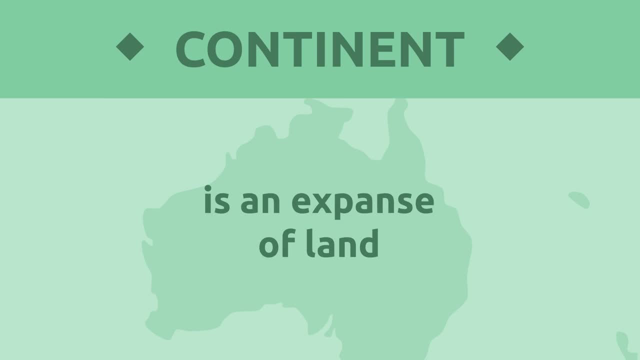 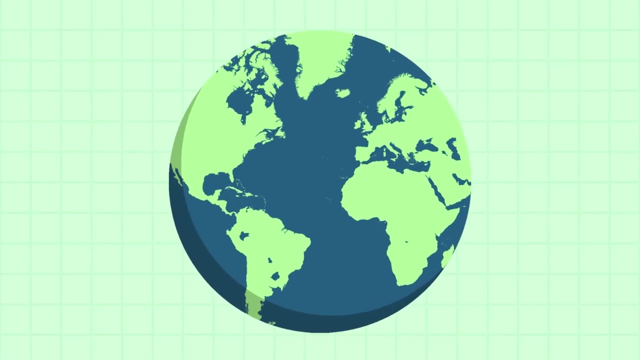 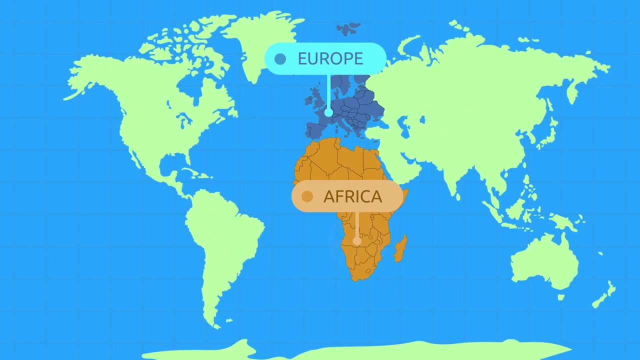 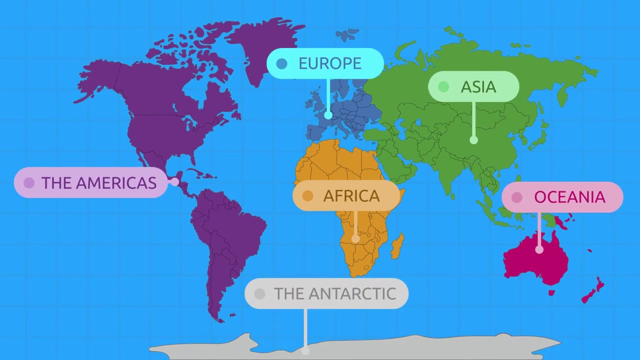 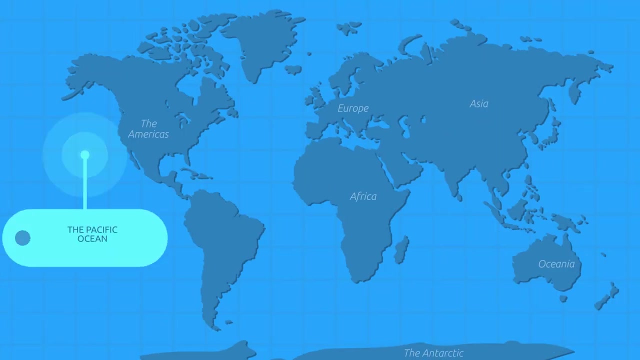 A continent is an expanse of land which is geographically and culturally differentiated from other continents. There are six continents on our planet: Europe, Africa, Asia, the Americas, Oceania and the Antarctic. These six continents are separated by five oceans. 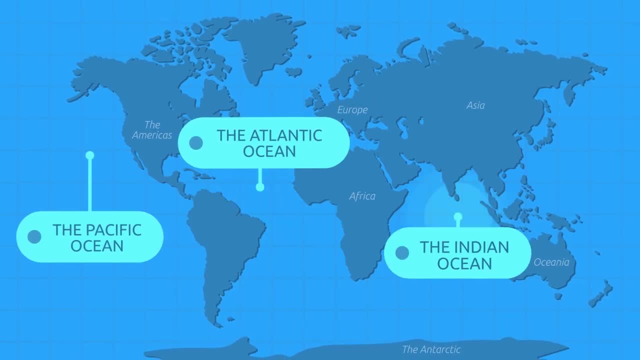 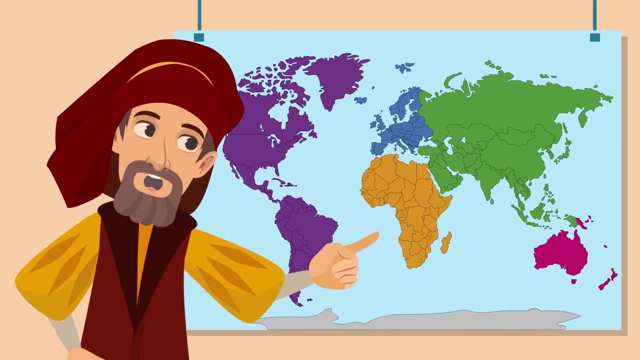 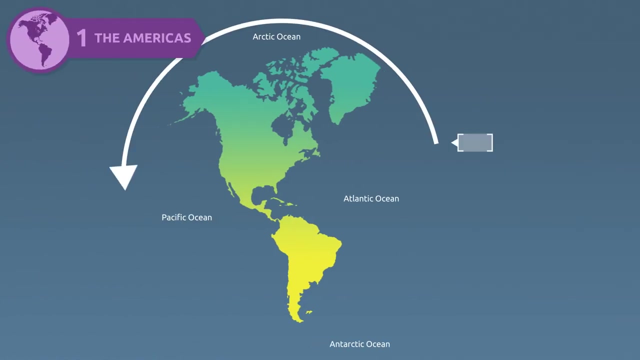 The Pacific Ocean, the Atlantic Ocean, the Indian Ocean, the Antarctic Ocean and the Arctic Ocean. Let's have a closer look at each one of these continents. The Americas: Owing to its size, geographical features and cultural characteristics, this continent 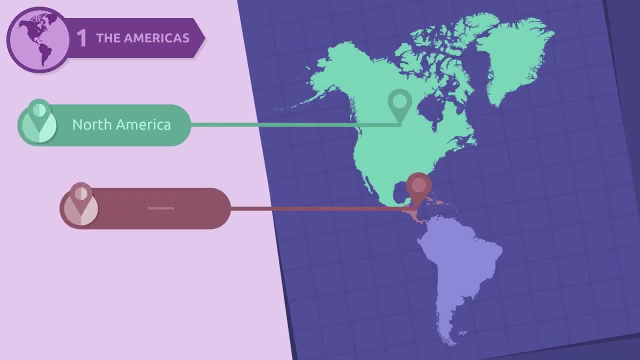 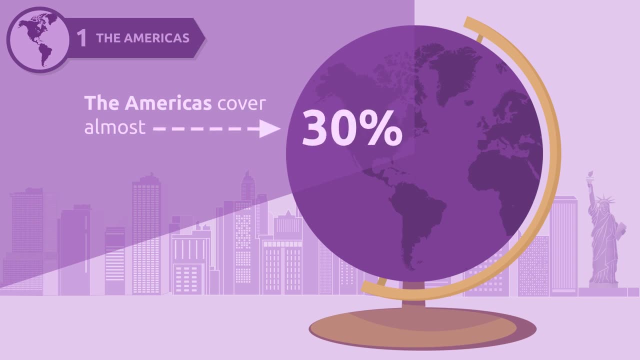 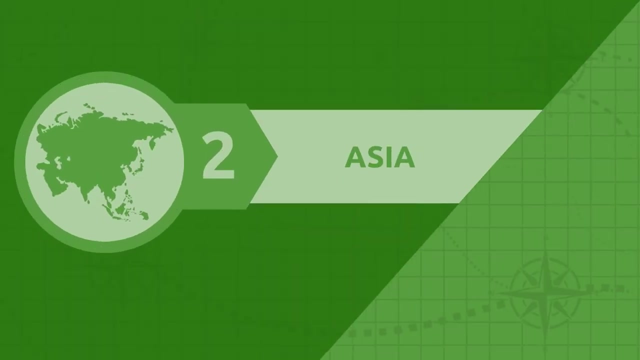 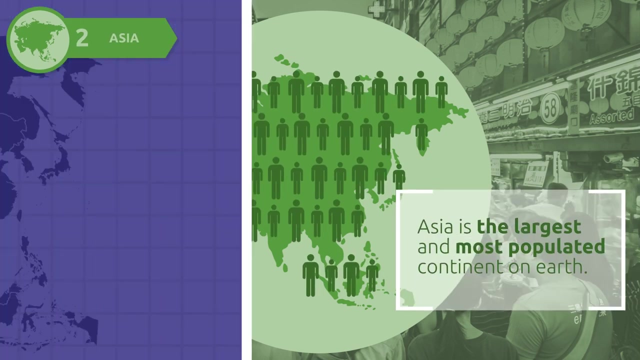 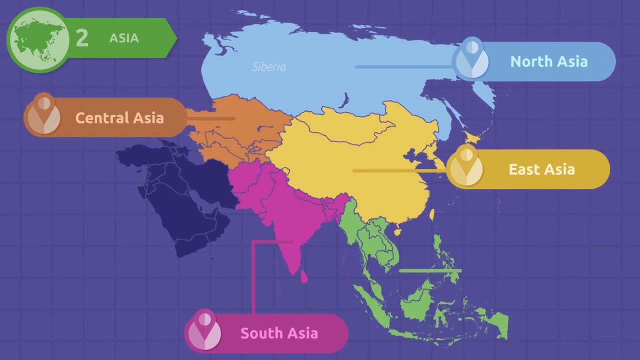 is divided into North America, Central America and South America. The Americas cover almost 30% of the Earth's total land area. The Americas, Asia, Asia- Asia is the largest and most populated continent on Earth. It is divided into North Asia, South Asia, East Asia, Central Asia, Southeast Asia and. 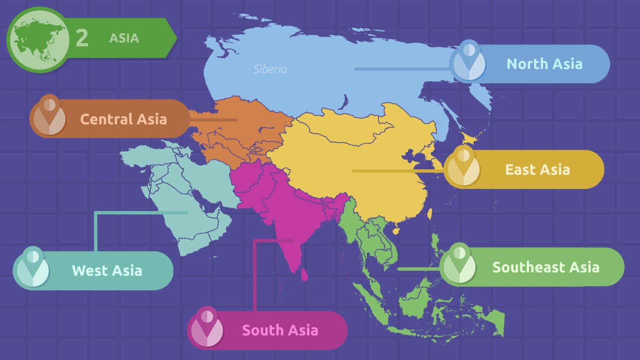 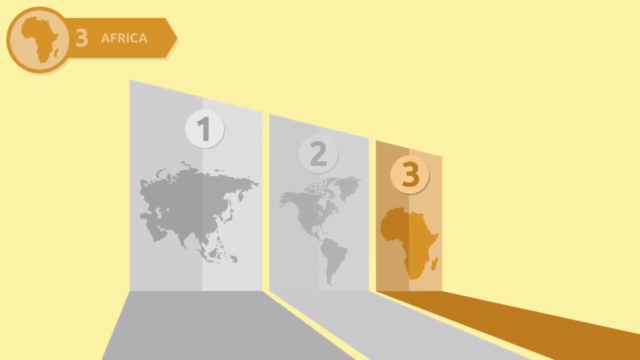 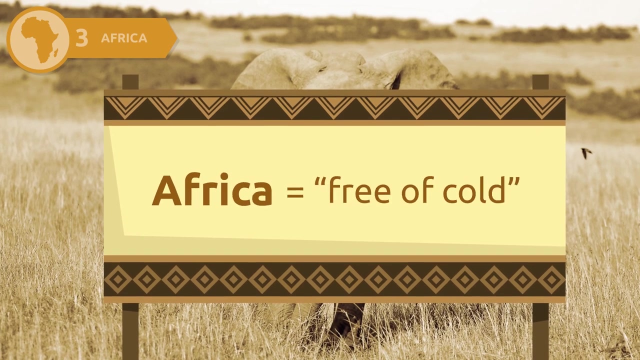 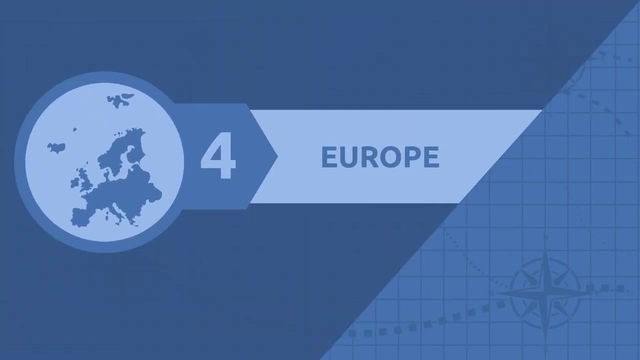 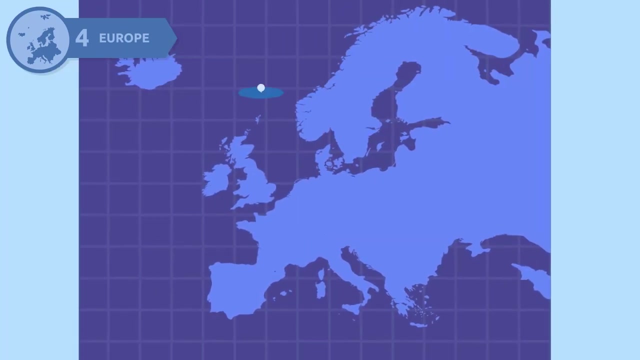 West Asia, Asia, Africa. Africa is the third largest continent in the world, after Asia and the Americas. The word Africa comes from Latin. It means free of cold Africa, Europe. Europe is also known as the Old Continent and is bordered by the Arctic and Atlantic. 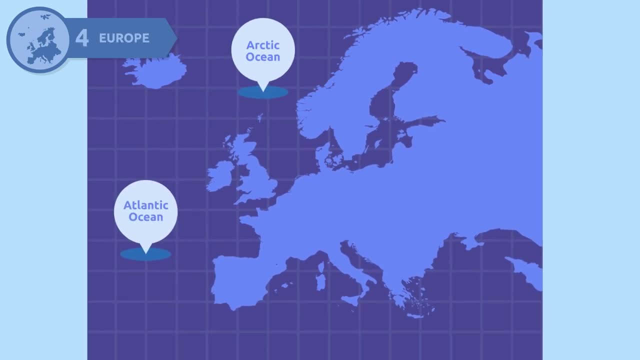 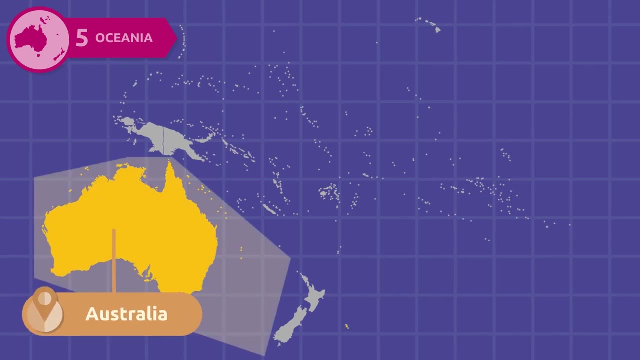 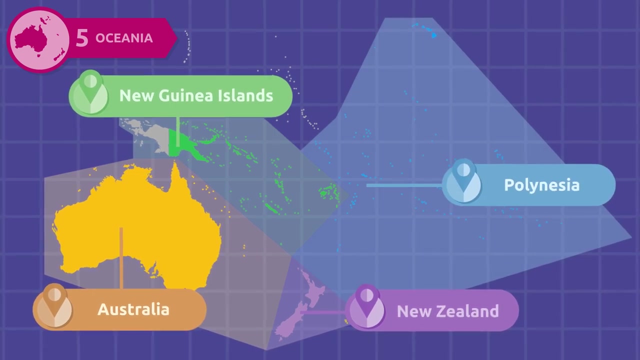 Ocean, Europe, Oceania. Oceania is made up of the island of Australia, New Guinea Islands, New Zealand, Australia, New Guinea Islands, New Zealand and several archipelagos like Polynesia. Oceania is surrounded.